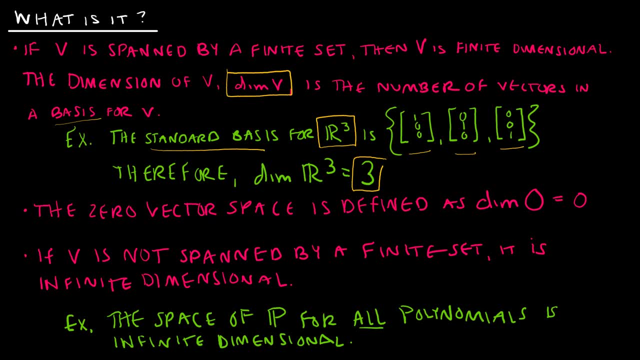 the number of vectors in the basis, If you have the 0 vector, space that is defined as 0. And if V is not spanned by a finite set, it's called infinite dimensional, and an example of that would be the space of all polynomials. So the space of P for all polynomials is infinite. 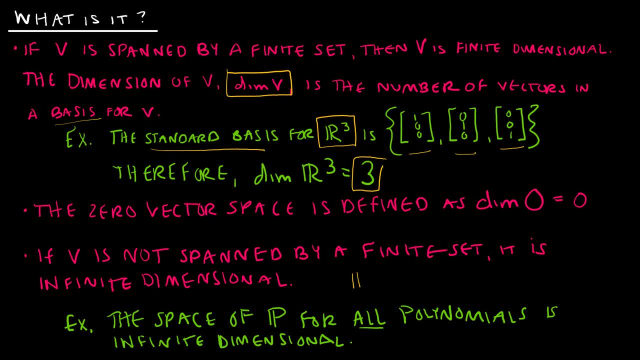 dimensional. Now, if I said just the space for P3, for instance, well then we could have a number, because P3, if you'll recall, would be 1, and then T to the first and T to the second and T to the. 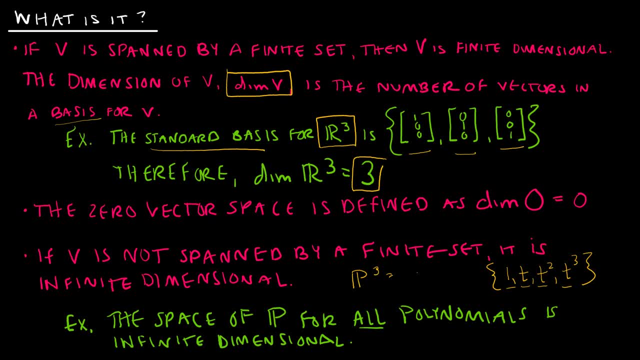 third, and this is 4.. And similarly, I could say P to the N would be N plus 1, because that same pattern is always going to hold, true, But for P3, for instance, well then we could have a number. 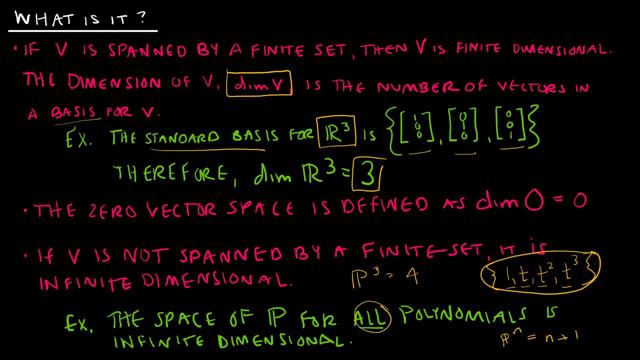 for the space of all polynomials. that would include P0, P1,, P2, P3, P4, all the way to infinity, and that's why that would be infinite dimensional. We're not going to really talk about this. 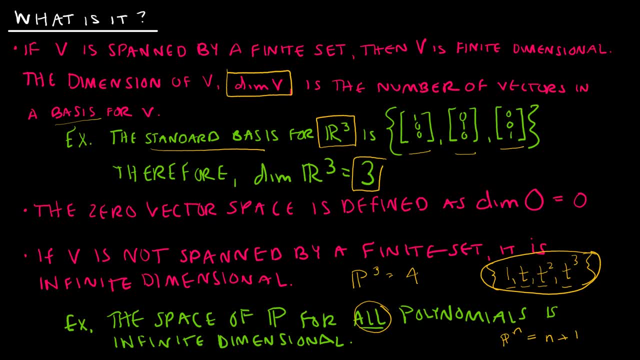 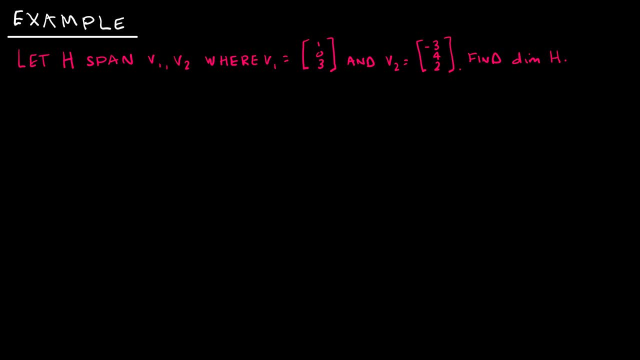 but I just wanted to point out that it's a thing that we're not going to do. Let's start out with a super easy example. I have two vectors here, V1 and V2, that is, we're saying H is the span of those vectors. 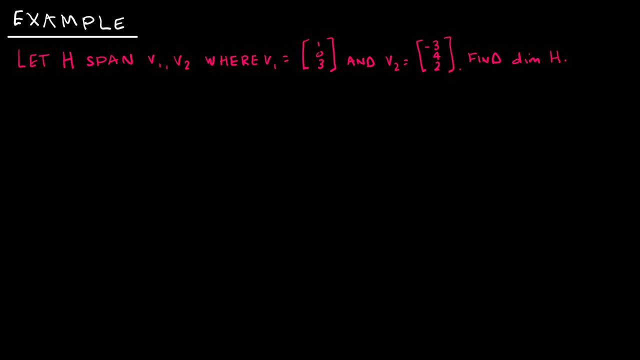 So if I have a vector that's a space of all polynomials, I'm going to say H is the span of those vectors. So I'm trying to find the dimension of H. So really, all I have to check in this case is: is it a basis, Which means, are these linearly independent? So therefore I'm just checking. 103. 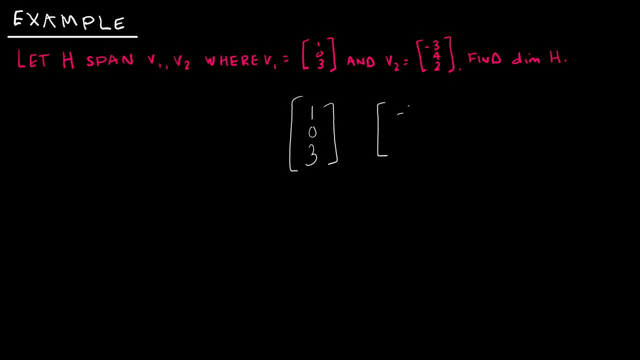 and checking negative 342, and those are not multiples of one another. So these two are linearly independent, And that's what we need for a basis. So of course the basis is 103, negative 342.. And therefore the dimension of H is two, because there are two vectors. Now I didn't do any work. 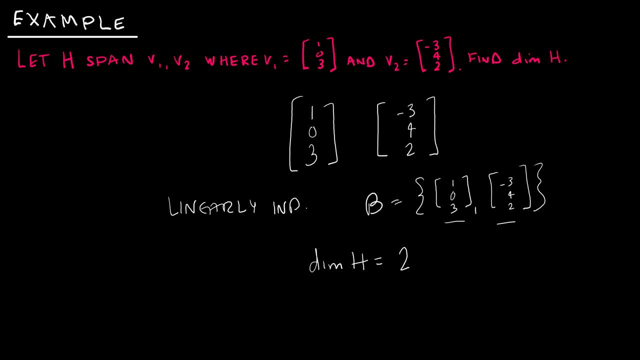 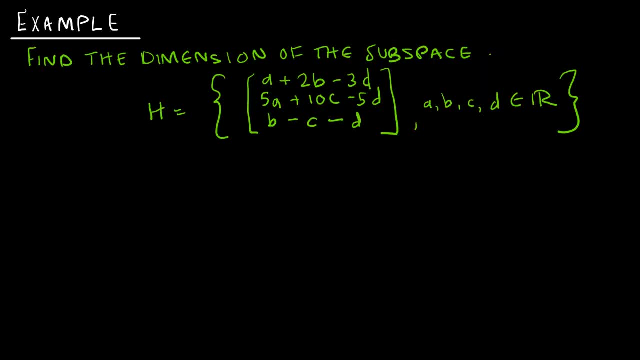 do a little bit of math to determine this. Let's take a look at a more difficult example, This: we have H and we're trying to find the dimensions of the subspace. So, again, all we're trying to do is determine how many vectors are in the basis of this subset H. And to start that, I would just 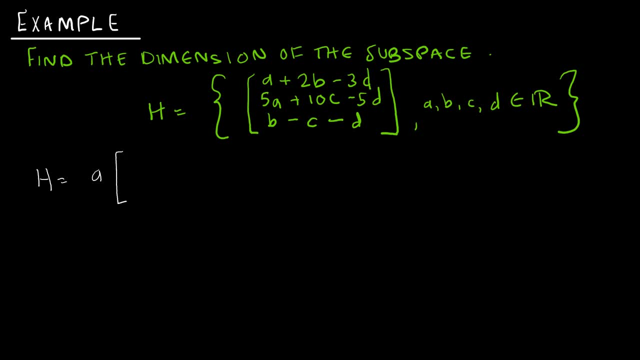 do some rewrites. So I'm going to take A and say there's one, five and zero. So I'm just going to taking those coefficients: one, five, zero. B would be two, zero one. C would be negative three. 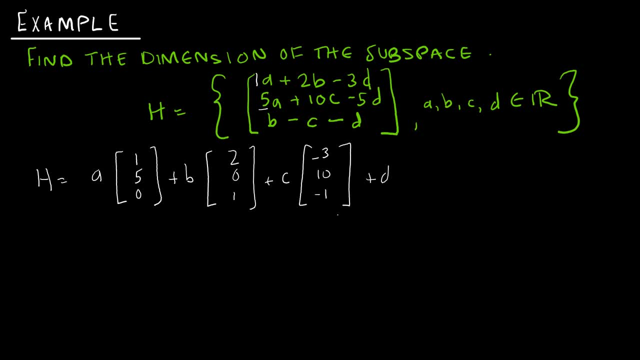 ten, negative one And D would be negative. three negative five. whoops, this was not negative three, that's zero. Negative three, negative five, negative one. So that's what I have for H. And remember, I don't care about the A, B, C, D. I care about the A, B, C, D, I care about the A. 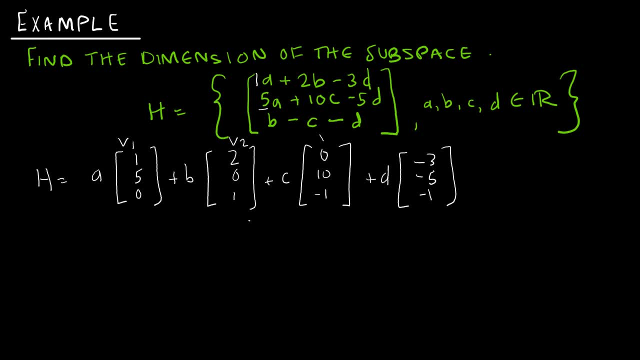 B, C, D- I care about those vectors- which is V1,, V2,, V3, and V4.. So essentially, what I'm trying to do is determine: are any of these vectors, can they be written as a linear combination of? 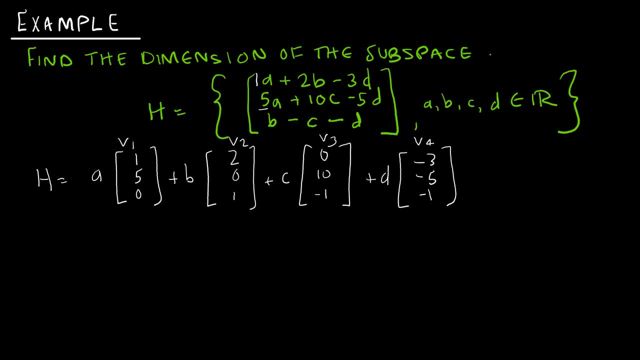 other vectors. So do I have any redundant vectors? So I'm going to essentially put these all together And you might be able to tell without doing any work, like we did on the last question. but quite often you're not going to be able to, So I'm going to show you what happens. 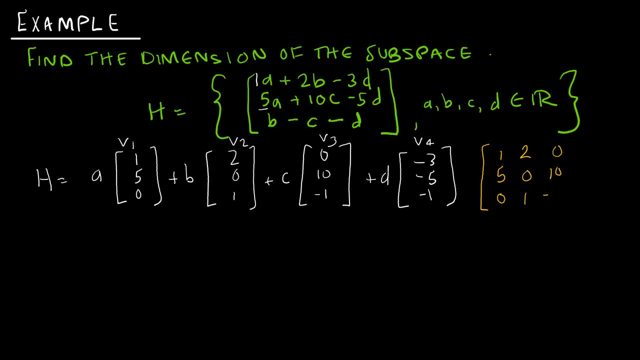 when we actually do that. I'm putting these all together into a matrix And I'm just going to do row operations to turn this into reduced row echelon form. That's going to give me 1,, 2,, 0, negative, 3. Negative: 5 times. 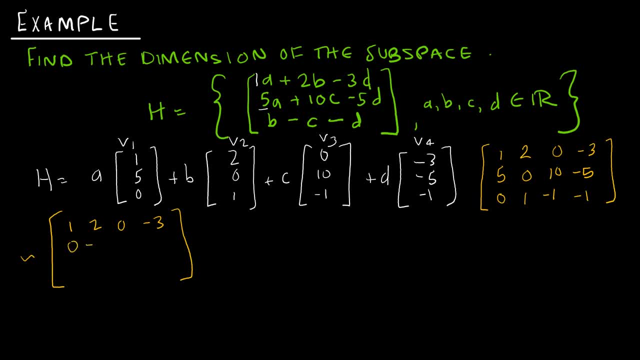 row 1 plus row 2 gives me 0, negative 10, positive 10, positive 10.. And row 3 doesn't change: 1, negative 1, negative 3.. And I'm just going to do row operations to turn this into reduced row echelon. 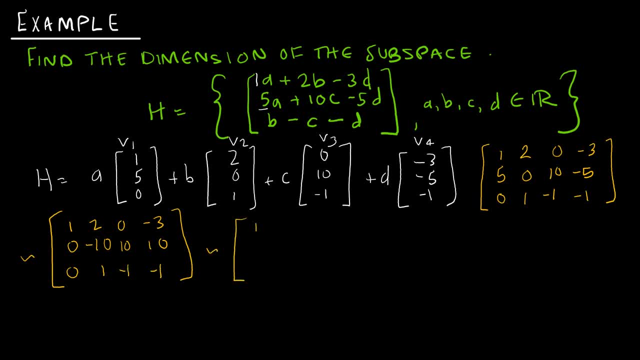 form. I'm going to set the number of vectors: zero plus zero plus zero plus one plus negative 1.. And my next step: I'm keeping row 1 the same. I'm keeping row 2 as negative, 1 on the right as negative, 1 on the left. 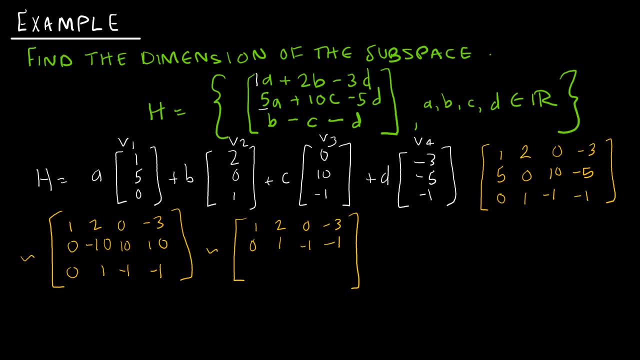 I'm keeping row 2 as negative: 1 tenth of the fifth row times row 2, which is 1, negative, 1, negative 1.. And I can see that if I took 1 tenth of row 2 and added it to row 3,. 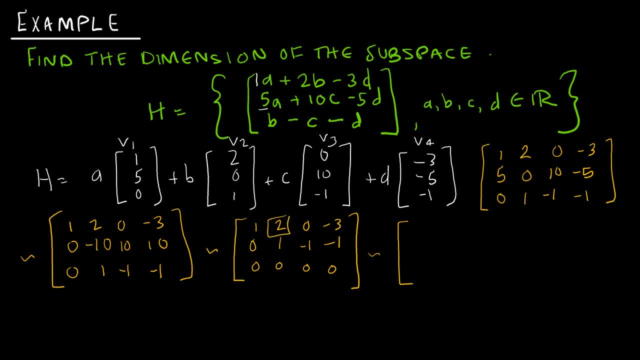 I would get 0, 0, 0, 0.. And I'm going to do just one more step because I want this guy two and add it to row one. Oops, that's still a one. And then negative two times one plus positive. 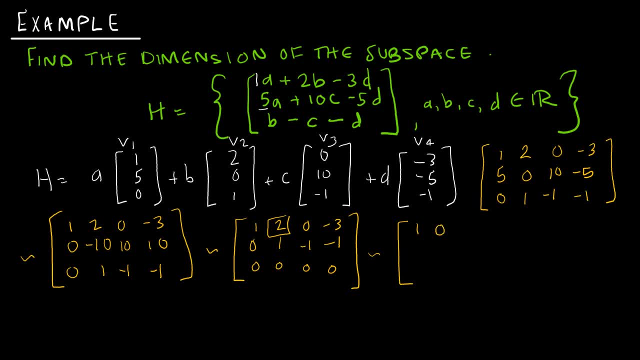 two Negative, two times negative, one is positive, two plus zero And negative two times negative. one is two plus negative, three is negative one, And then I have zero, one, negative one, negative one, zero, zero, zero, zero. So now what I'm trying to determine is: are any of these 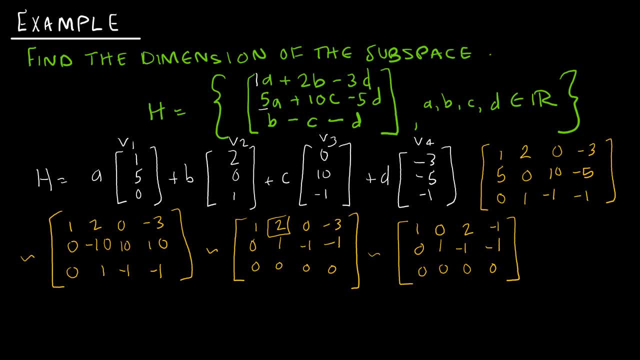 linear combinations of others. So I've got: V1 is one zero zero and V2 is zero, one zero. So clearly those are fine. They are not linear combinations of others. But it looks like for V2,, X2, and V3, there's no linear combinations of others. So I'm trying to determine. 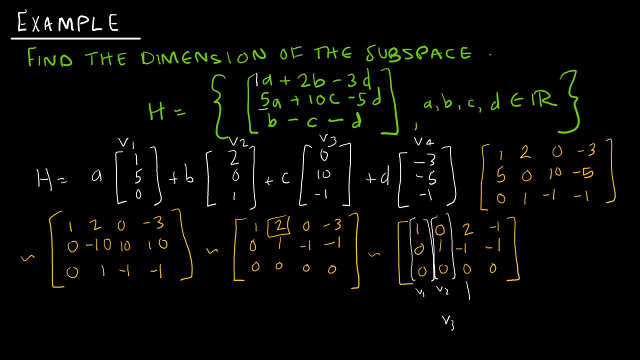 so clearly. those are fine. They are not linear combinations of others, But it looks like for V1, V3, I could write it as a linear combination of V1 and V2.. So if I took 2V1 and I subtracted V2, 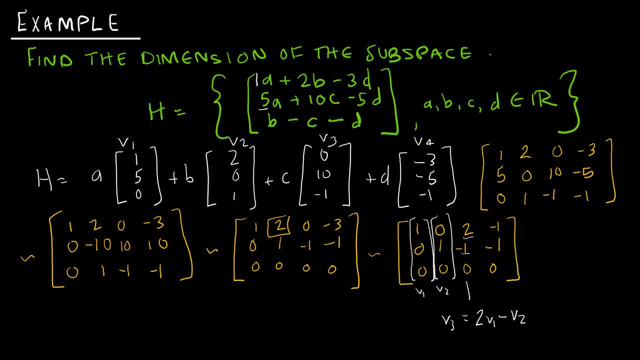 so 2V1 and I subtract V2, which gives me 2, negative, 1, 0. Therefore, R3 is a redundant vector And remember, using the spanning set theorem, I can remove it. So it's not going to. 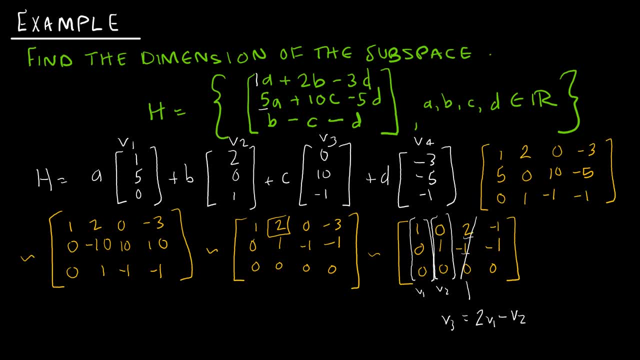 be part of the basis. And then if I look at V4, V4 can be written as negative V1 minus V2. Because again, that would give me negative 1, negative 1, 0. And I can just for fun.